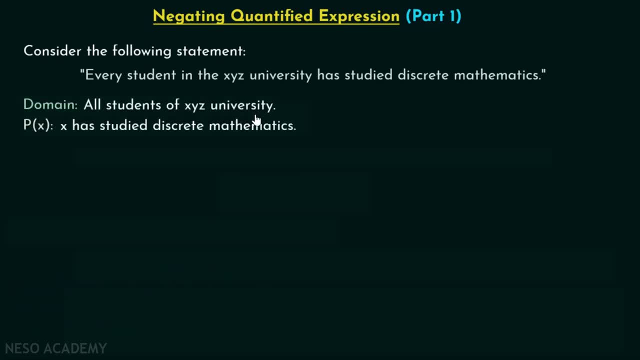 For this purpose, we will consider the domain as all students of XYZ university. This is my assumption. I am considering the students of XYZ university only, Although I can also consider all students of every university known in this world, But here, in this case, I am considering the domain. 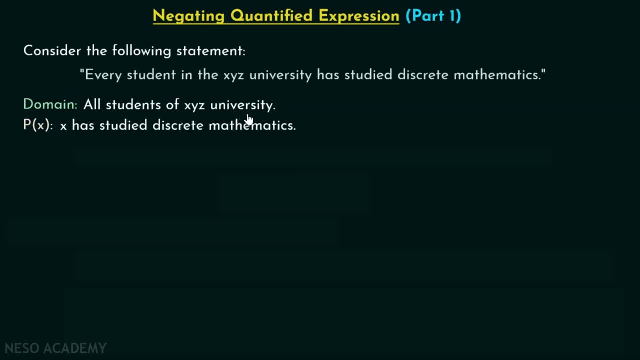 as all students of XYZ university. This will simplify the process a bit. Now we shall also consider Px, which denotes X has studied discrete mathematics. Okay, so Px is a predicate that denotes X has studied discrete mathematics. We can rewrite this particular statement, that is: 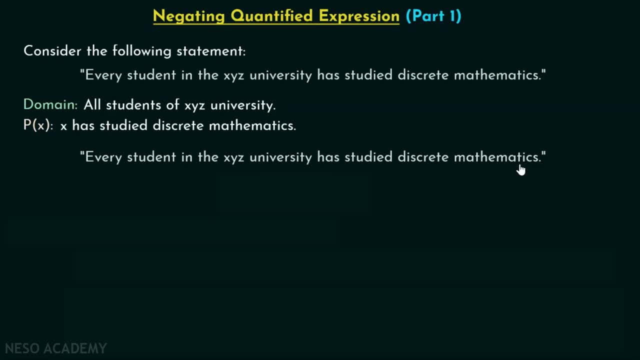 every student in the XYZ university has studied discrete mathematics, as for all X Px, Isn't that so? It becomes easier because here we know every student in the XYZ university has studied discrete mathematics, which means for all X- Px. We are considering Px as X has studied discrete mathematics. 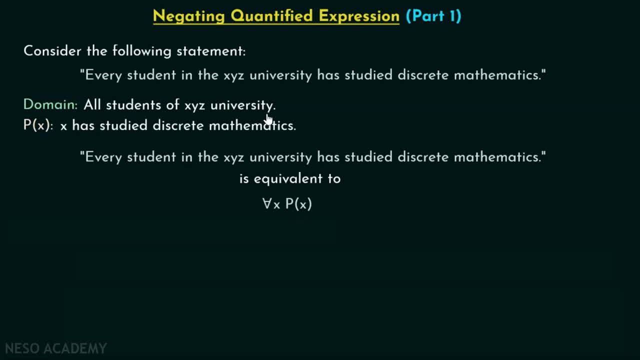 and we know we are considering this domain. that is, all students of XYZ university, So we can rewrite this statement. as for all X Px, Let's try to find out what is the negation of this particular statement. It is not the case that. 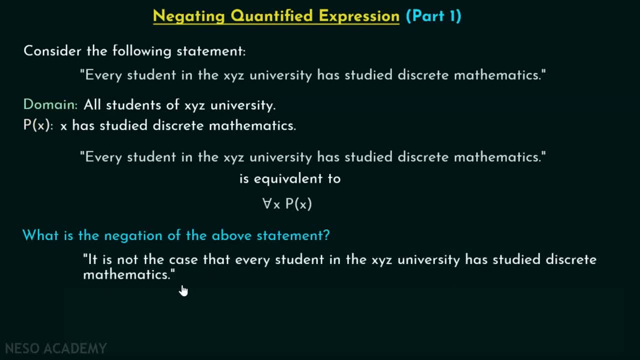 every student in the XYZ university has studied discrete mathematics. This is the negation of this particular statement. Just put this particular line, that is, it is not the case that in front of this particular statement, Then it becomes negation of this statement. We can also write this in a better form: 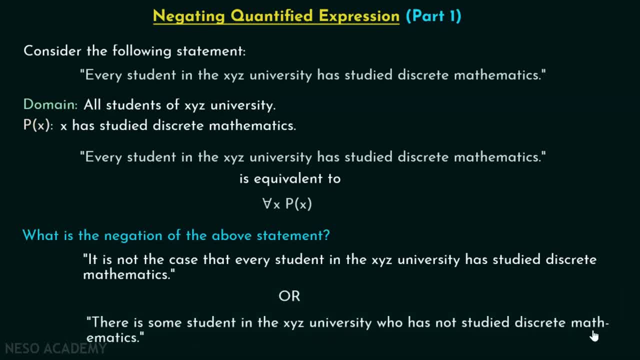 that is, there is some student in the XYZ university who has not studied discrete mathematics. Understand this. Here I am considering the statement: every student in the XYZ university has studied discrete mathematics. We need to find the negation of the statement, that is, we need to complement. 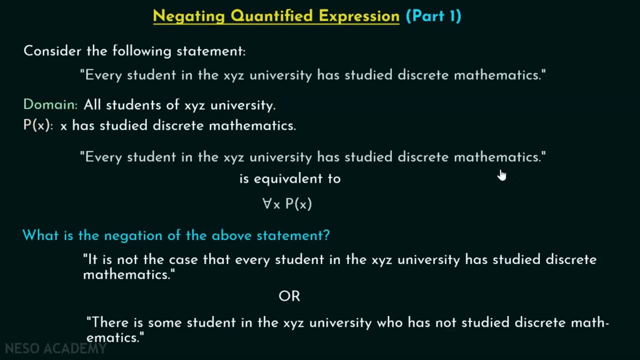 this statement. Isn't that so, Which means this is just opposite of that? Now understand this. What is the opposite of the statement? There is some student in the XYZ university who has not studied discrete mathematics. Of course there must be at least one student. 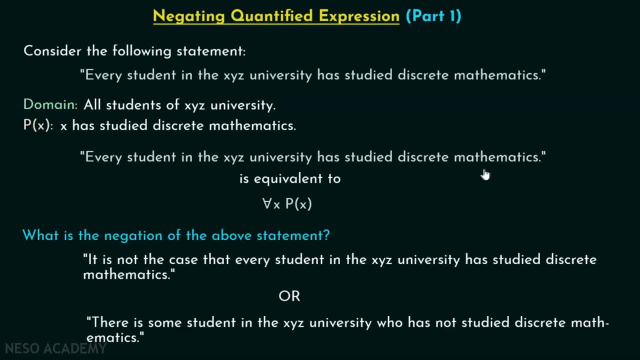 in the XYZ university who has not studied discrete mathematics, That particular statement will be the complement of this statement. Isn't that so? Because here I am considering, every student in the XYZ university has studied discrete mathematics. If there is just one student in the XYZ